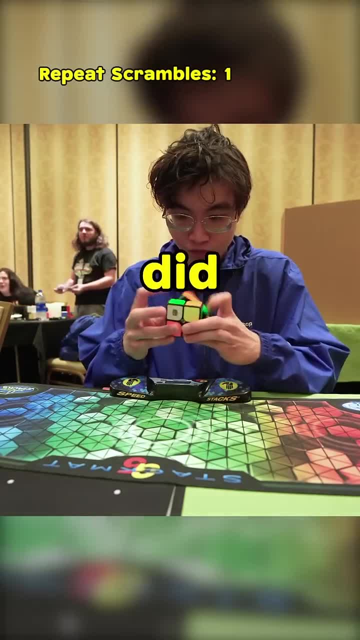 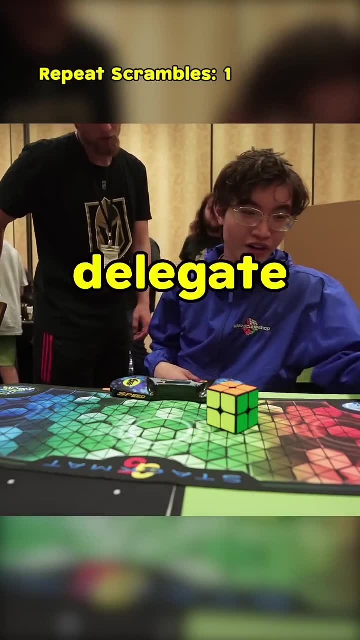 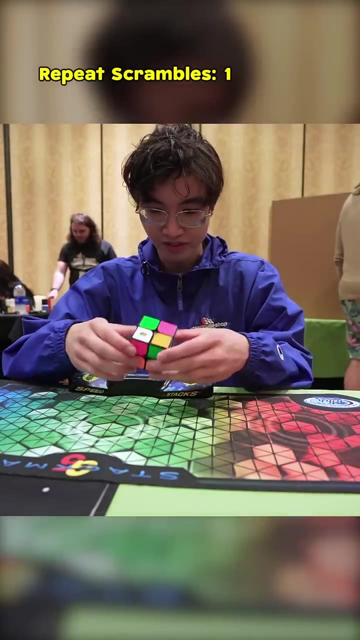 familiar. I immediately recognized it. but I did the solve to confirm if I would get the same solution, which I did. And then I told my judge and called a delegate to review. They gave me another scramble to review and it was the same again. I told my delegate and got a new one that was correct. 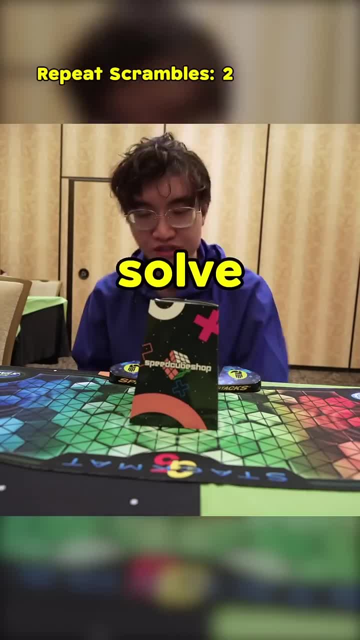 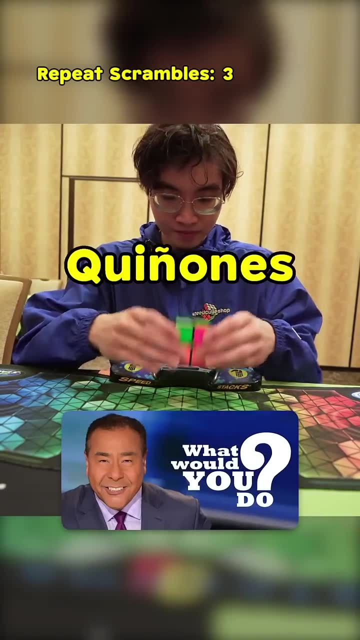 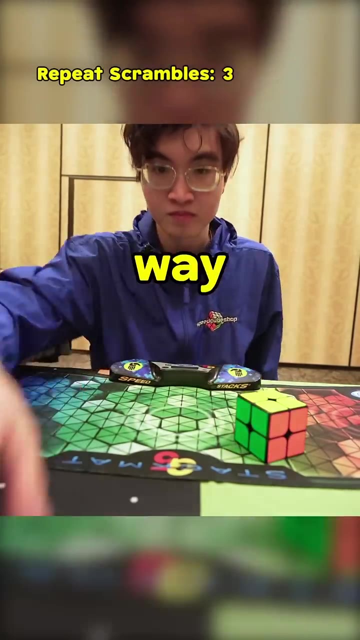 But the story does not end there. On my fifth solve, look at this Same scramble again. At this point I am looking for cameras, if anyone is testing me, like John Quiones with his tv show, I could have had one second solved if I did not spoken up. The scramble was that good, but honesty is the way to go. 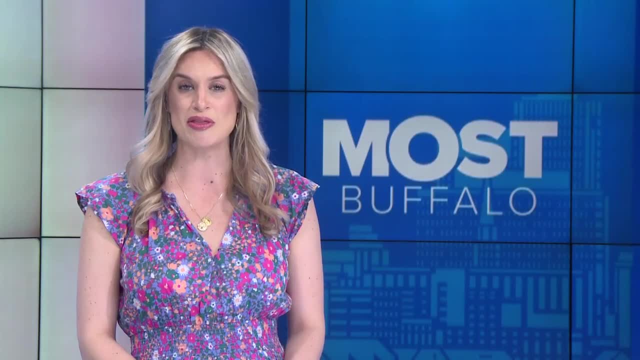 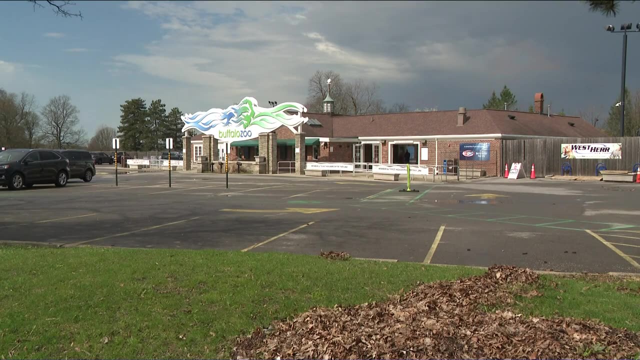 But first a follow up to a story we brought you last Thursday about the Buffalo Zoo increasing their prices Most Buffaloes. Andy Payton joins us from the zoo with exactly how much it will cost you to park and get in this spring and summer. Hi, Andy. 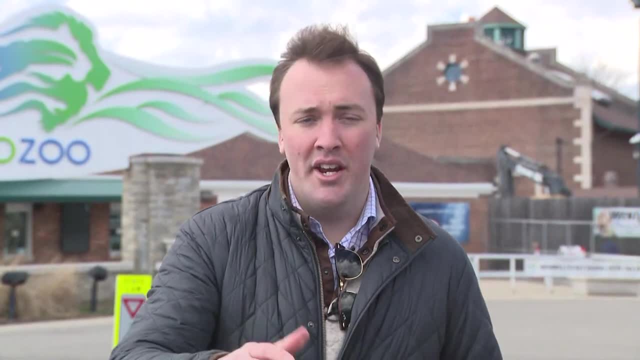 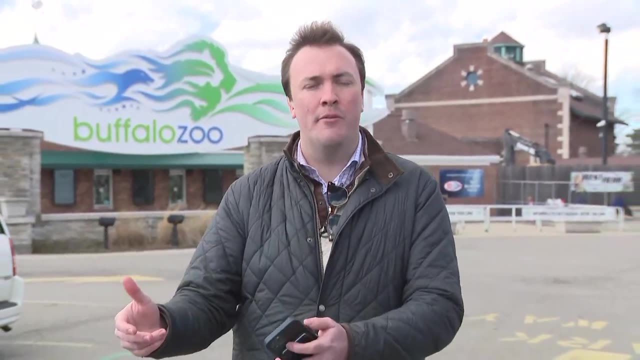 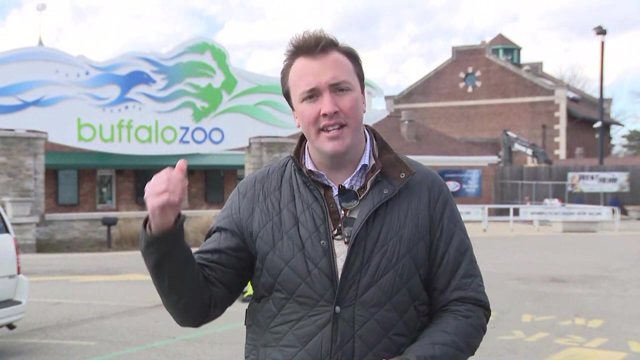 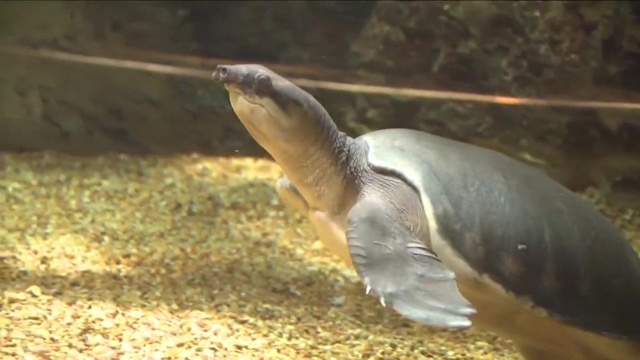 Hey there, Lauren, That's right, You know. we're right outside the Buffalo Zoo here. It just closed a few minutes ago and today marked the first day that those new prices went into effect for admission. just a few weeks ago, or actually just last week In fact, it was 1795 for an adult ticket to get inside the Buffalo Zoo, But today it is now around $22 for admission, and that's only going to go up because we're in the off season period right now. in late May, around May 25th is when the end season period kicks in and that's when you're going to see the prices go up. 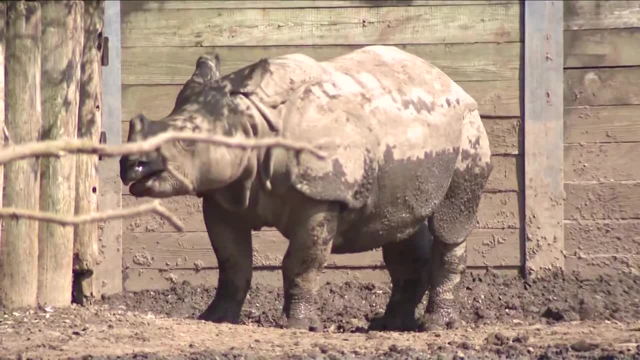 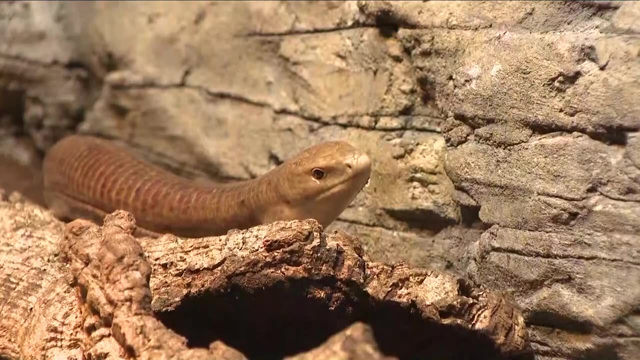 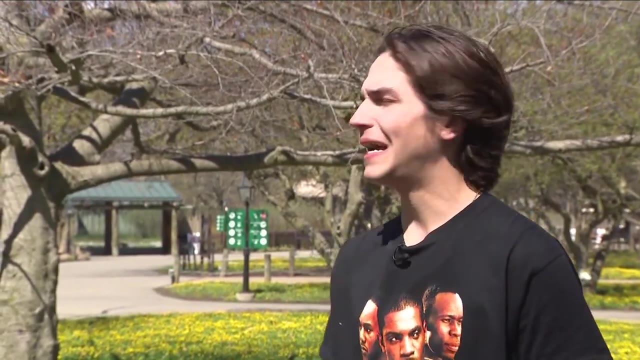 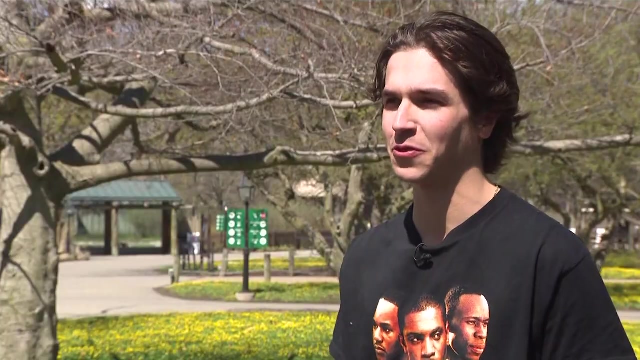 So you're going to see a ticket for an adult at about $26.. Now we spent the past few hour and an hour and a half So here talking to some zoo goers about the new prices And, as you can imagine, they weren't too pleased about it. Take a listen to this. Do you think it? do you think it's worth being the most expensive zoo? I would say not. Unfortunately, I haven't seen enough, But from what I've seen, I don't think it's $26 worth. Oh, it's too high because for for a student it's to pay $22..